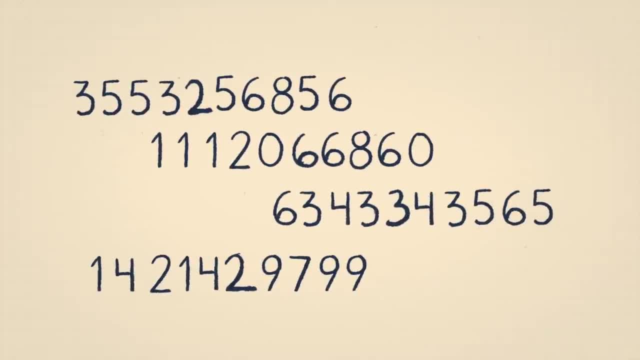 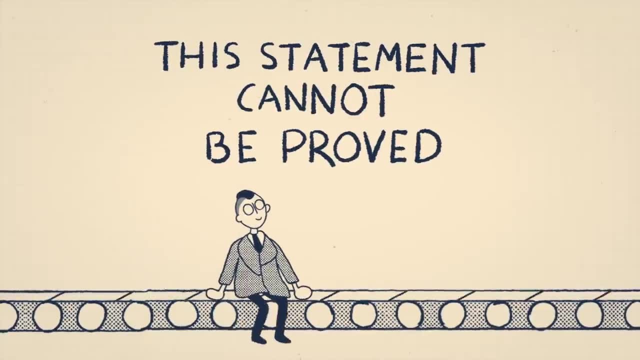 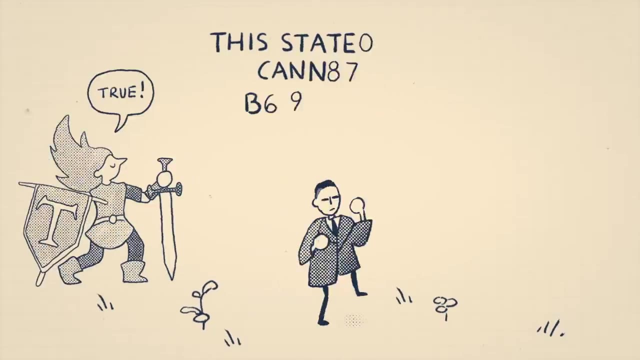 In this way, the coding allowed mathematics to talk about itself. Through this method, he was able to write. this statement cannot be proved as an equation, creating the first self-referential mathematical statement. However, unlike the ambiguous sentence that inspired him, 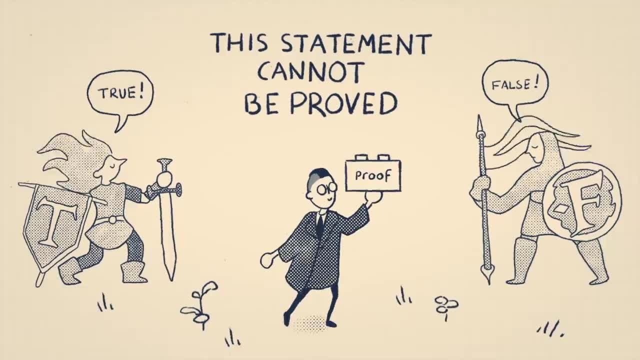 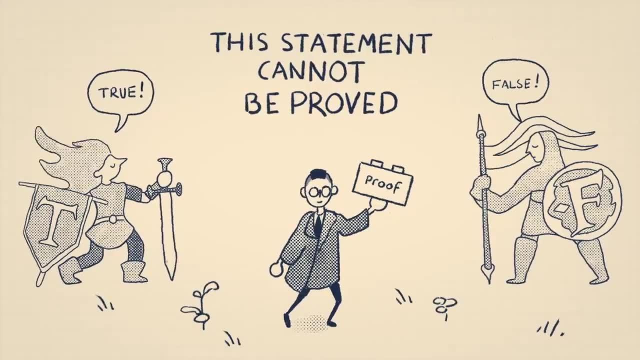 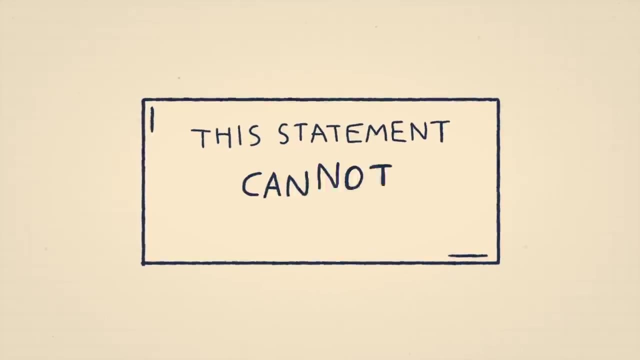 mathematical statements must be true or false. So which is it? If it's false, that means the statement does have a proof. But if a mathematical statement has a proof, then it must be true. This contradiction means that Gödel's statement can't be false. 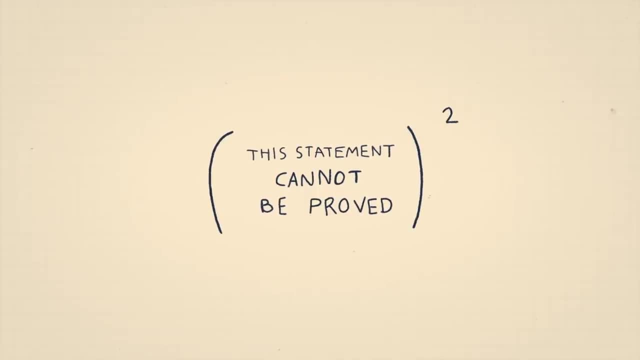 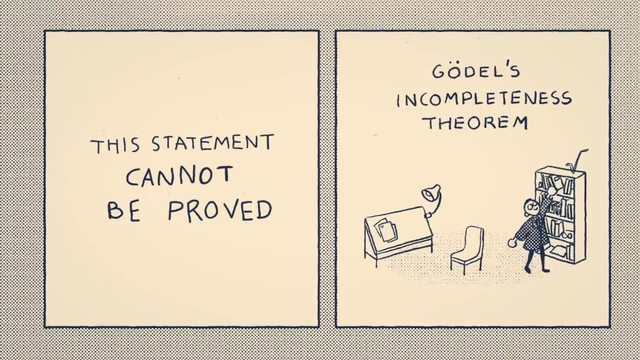 and therefore it must be true that this statement cannot be proved. Yet this result is even more surprising because it means we now have a true equation of mathematics that asserts it cannot be proved. This revelation is at the heart of Gödel's incompleteness theorem. 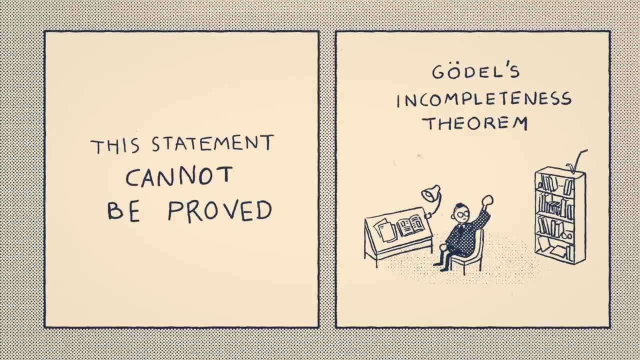 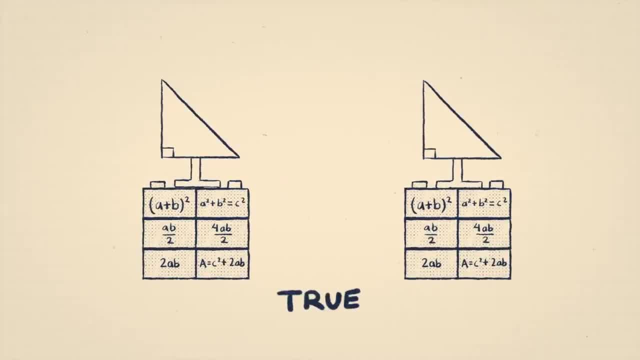 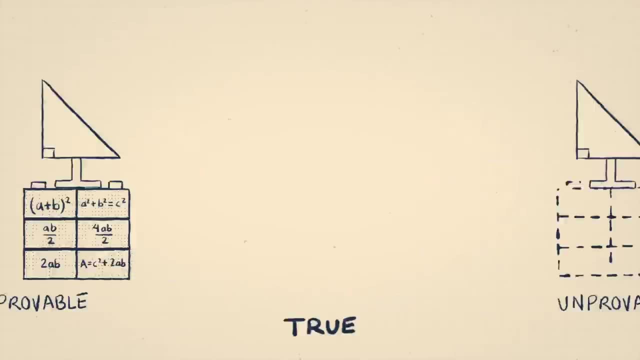 which introduces an entirely new class of mathematical statement. In Gödel's paradigm, statements still are either true or false, But true statements can either be provable or unprovable within a given set of axioms. Furthermore, Gödel argues, these unprovably true statements exist in every axiomatic system. 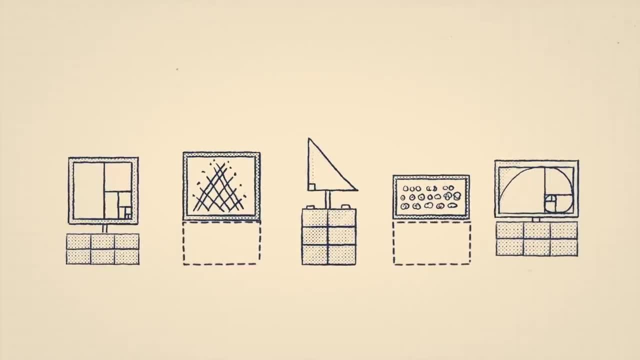 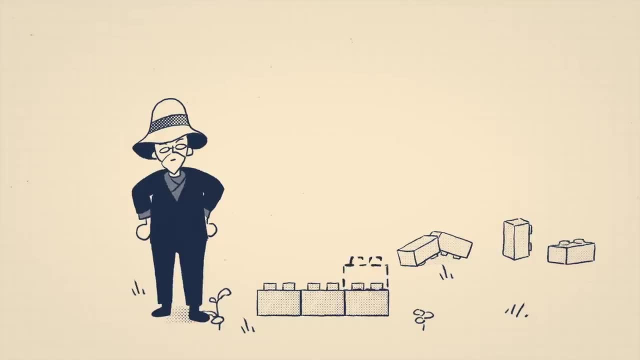 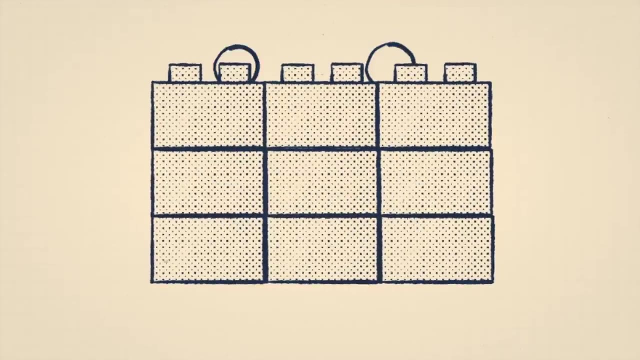 This makes it impossible to create a perfectly complete system using mathematics, because there will always be true statements we cannot prove. Even if you account for these unprovable statements by adding them as new axioms to an enlarged mathematical system, that very process introduces new, unprovably true statements. 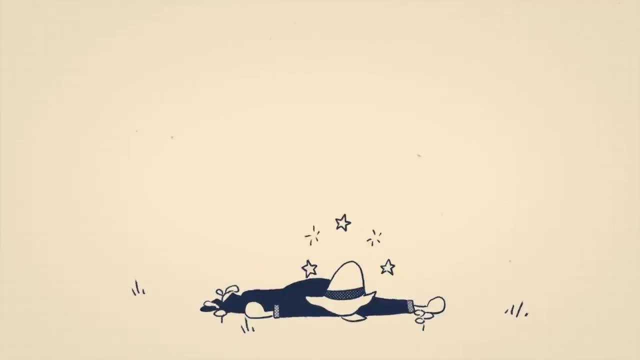 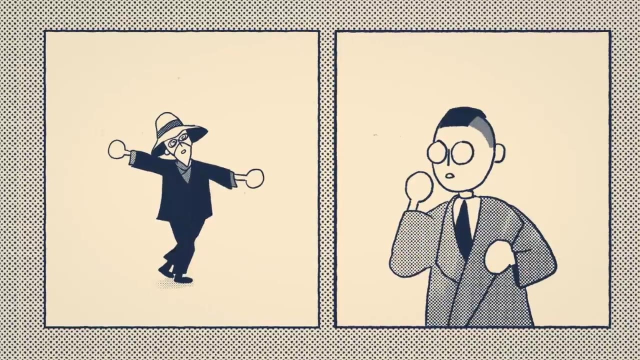 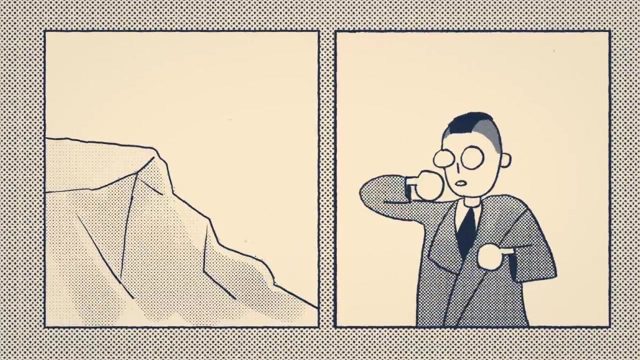 No matter how many axioms you add, there will always be unprovably true statements. in your system. It's Gödel's all the way down. This revelation rocked the foundations of the field, crushing those who dreamed that every mathematical claim would one day be proven or disproven. 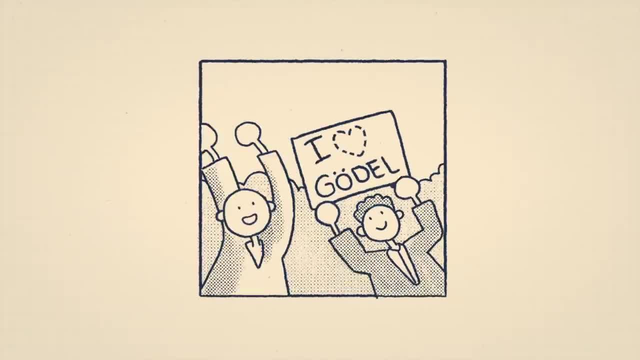 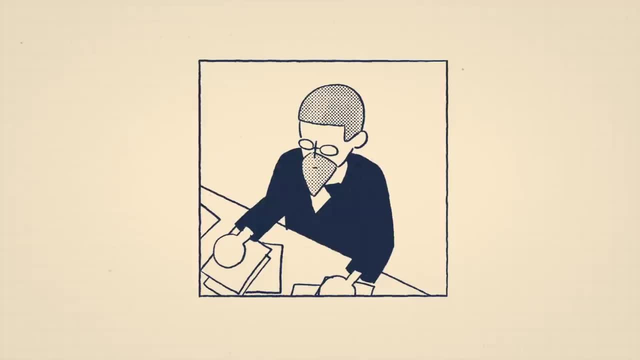 While most mathematicians accepted this new reality, some fervently debated it. Others still tried to ignore the newly uncovered hole in the heart of their field. But as more classical problems were proven, or proven to be unprovably true, some began to worry. their life's work would be impossible to complete.